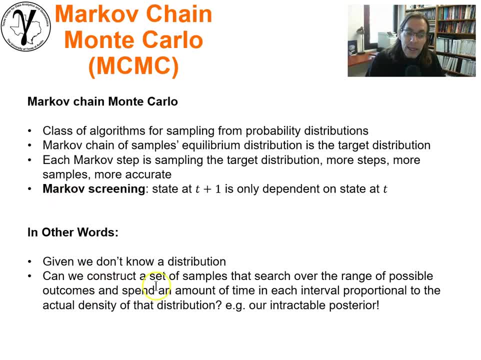 of possible outcomes, and we need it to be set such that it spends an amount of time in each interval within the possible solution space proportional to the actual density of that distribution. In other words, we're trying to get to a posterior with our Bayesian linear regression. 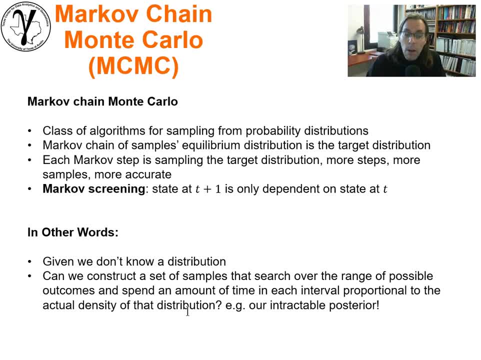 and we can't get directly to it for a continuous variable, but Markov chain, Monte Carlo. we're able to sample from that distribution. If we do enough samples, we'll actually know what the distribution is. Okay, that seems a little bit complicated. 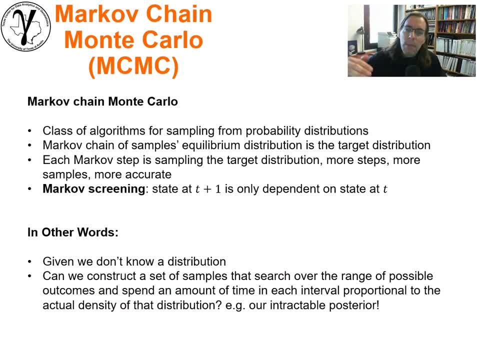 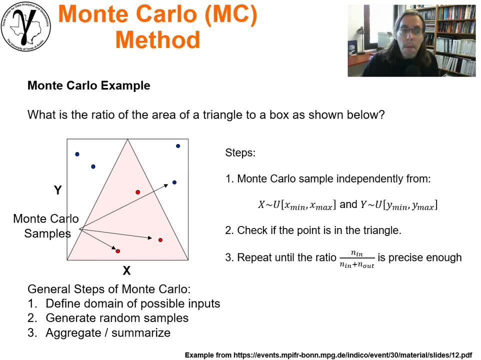 Let's go ahead and walk through. We'll step up towards that problem. Let's start with something very basic. Let's forget about Markov chains and let's just think about a very simple Monte Carlo method to solve a very simple geometric problem. 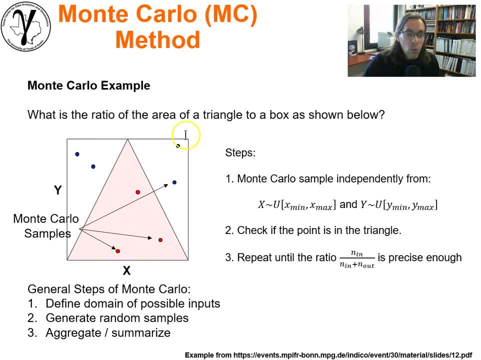 Okay, so we have this area of interest right here in x and y and we want to know what is the ratio of the area of the triangle to the area of the box. So we want to solve for the proportion of this box that is triangle. 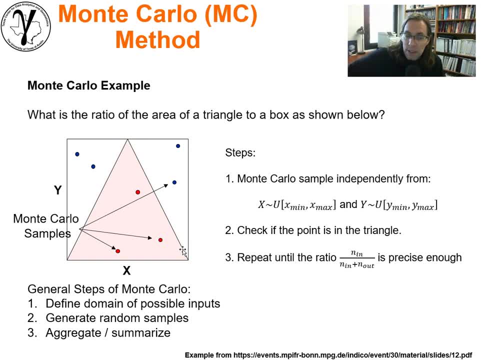 Okay, so what would be the Markov methodology to solve this problem? What we could do is we could do Monte Carlo, sampling independently from x and y. What would that look like? We would be sampling from uniform distributions, from x min to x max, y min to y max. 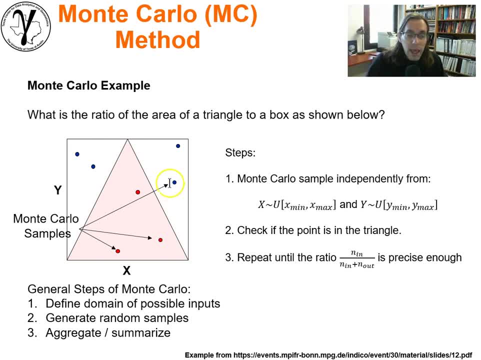 and if we do that independently, the result is we will get individual samples like these. I drew these as Monte Carlo samples and they'd be uniformly distributed on each axis. Now what we do next is we take that point and we check. 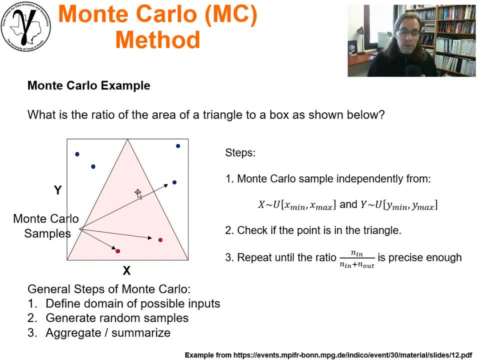 am I inside the triangle, If you are, turn it red, That's an in point. Or am I outside the triangle? Turn it blue? That's an out point. Now, I hope you can see that if I do that enough, 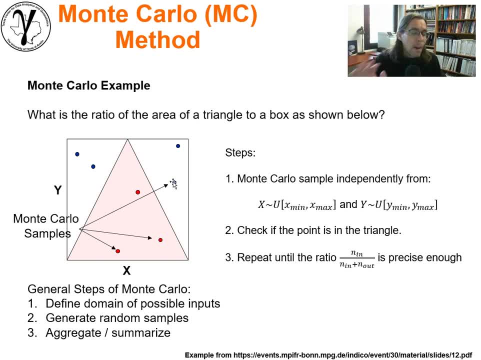 I do enough samples. I do a thousand, a million samples, ten million samples, and so forth. what will happen is my assessment of the area of the triangle as a proportion of the total area, as calculated as the number of points within the triangle. 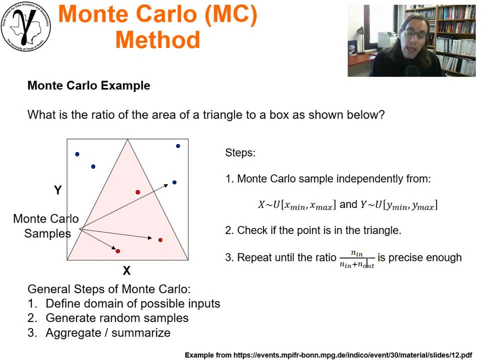 divided by all points in and out, that this will get very precise. This would become a very precise estimate. So what have we done? We solved this geometric problem, for which the only thing we could do was we could tell if a point was inside the triangle. 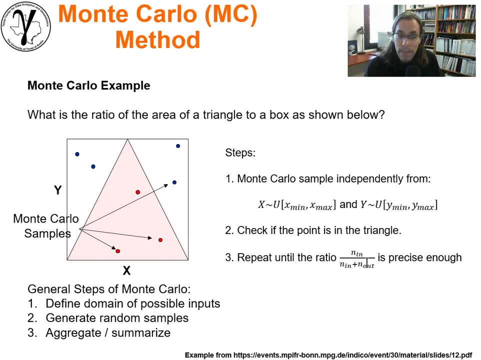 Never once did I have to calculate the area of the triangle, But by doing enough samples I got to the distribution, In this case just simply a proportion, and it was pretty straightforward. So the general steps of Monte Carlo define the domain of possible outcomes. 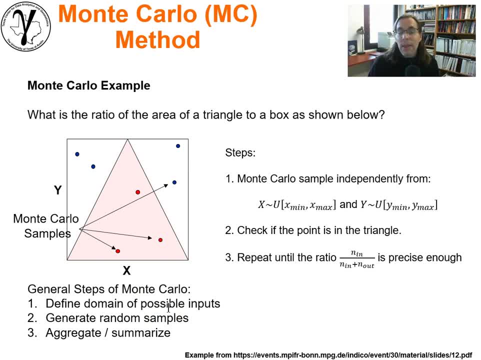 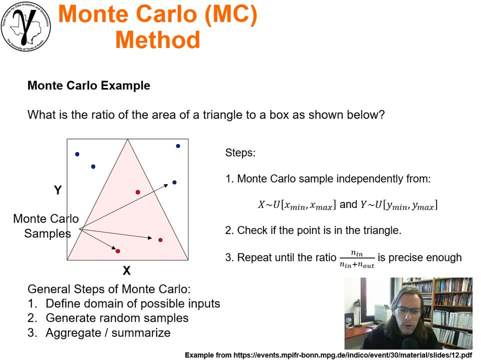 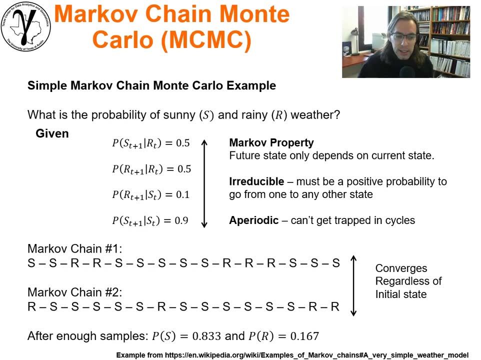 generate random samples and aggregate and summarize those results to get your answer. Now let's go one step further and look at the idea of Markov Chain, Monte Carlo. So let's take a really nice example right here. This example was taken from Wikipedia. 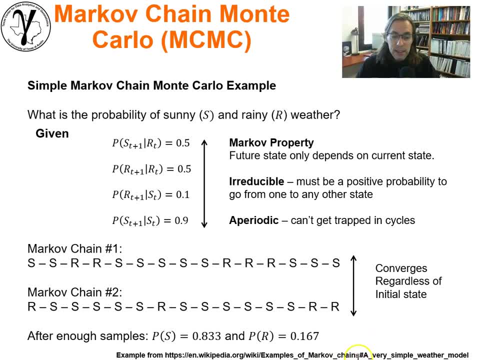 They have a really nice page on examples of Markov chains, And this is the very simple weather model, And so here's our problem right now. We have a sunny or rainy state from day to day, And we want to be able to calculate. 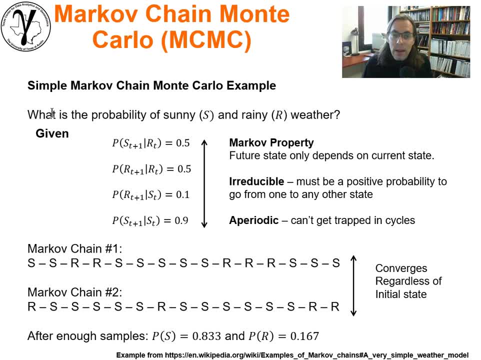 what is the probability of sunny or rainy weather, And all we have available to us are the following conditional probabilities: If it's raining today, it will be a 50% chance to be sunny tomorrow. If it's raining today, 50% chance of being rainy tomorrow. 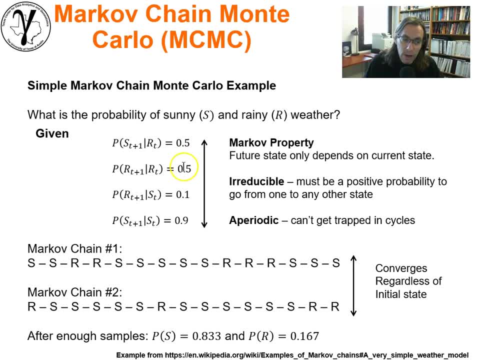 Oh, satisfies closure. That makes sense, right? 50-50, right? If it's sunny today, 10% chance of being rainy tomorrow and 90% chance of being sunny tomorrow if sunny today. So this is what we know. 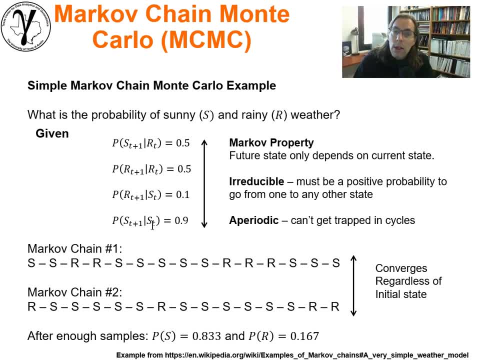 Now I don't know and I can't get to the global probability of sunny or rainy. I just know these conditional probabilities. Now they're Markov property, because they have a Markov property, because the future state depends only on the current state. 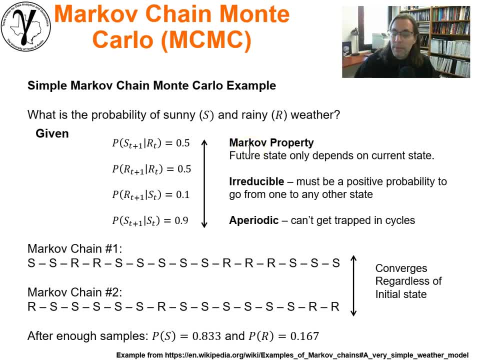 not information from way in the past. Tomorrow depends just on today. They're irreducible because every possibility, every transition has a probability of occurrence. So we're able to explore. You'll see, we'll be able to explore the problem very well. 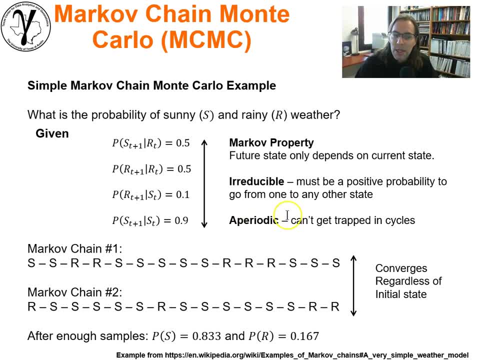 And they're aperiodic, periodic, because there's no getting trapped. We're not going to get trapped in sunny, It'll just be sunny. We won't just get trapped in rainy, It can go back and forth anywhere. There's no way to get trapped in the system. 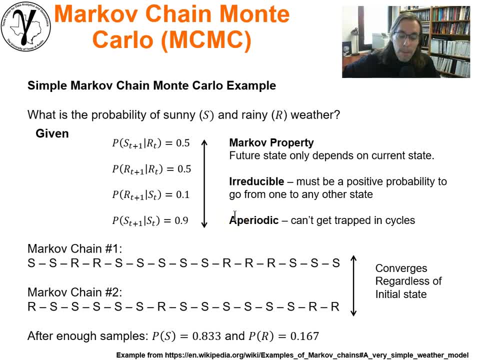 Okay, let's go ahead and do Markov chain Monte Carlo simulation. So step number one: pick a random state, Just pick one. This is categorical. We'll just pick rainy or sunny. Okay, sunny, sunny day today, That's good. 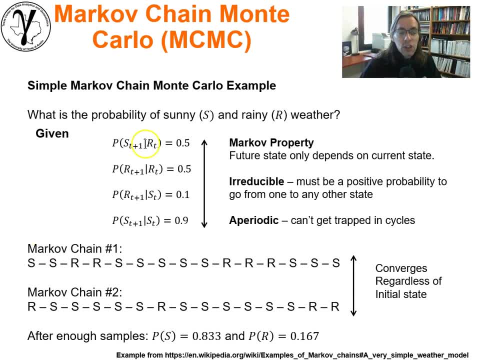 Love the sun, So we have sun. Now we go to the conditional probability. We want to do a Monte Carlo simulation to generate our chain, to keep our chain going, with its correlation, its structures as defined by these Markov properties and rules. 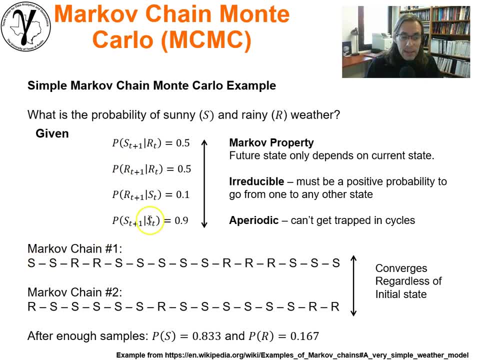 Markov rules. So we look: sunny day today, 90% chance of sunny sunny tomorrow. We do a Monte Carlo simulation sunny. We rolled the dice or we used a random number seed and we got a number less than 90%. 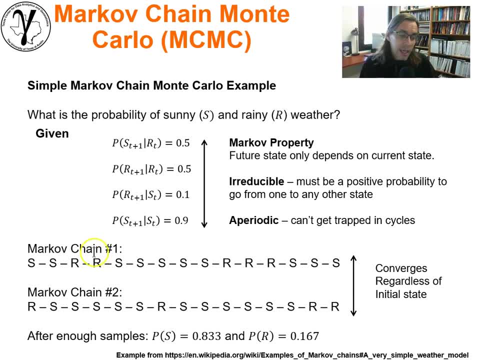 It's sunny. Okay, So sunny again. We do that. again It's sunny. We use the same rule again. Oh, we got something that's now rainy rainy. Oh, once it's raining, 50% chance of being raining. 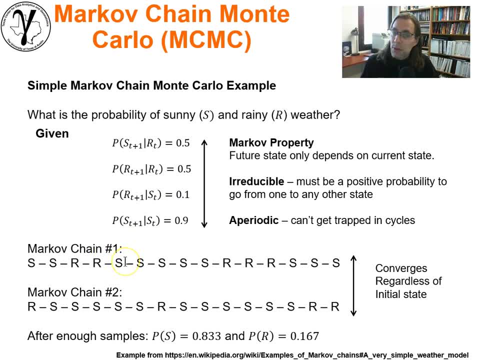 Okay, Raining again. Oh, 50% chance of sunny. It's sunny again: 90% chance of being sunny: 90%. You see what I'm saying, And we keep going long enough. These are going to be a nice set of samples from the global proportion that we're seeking. 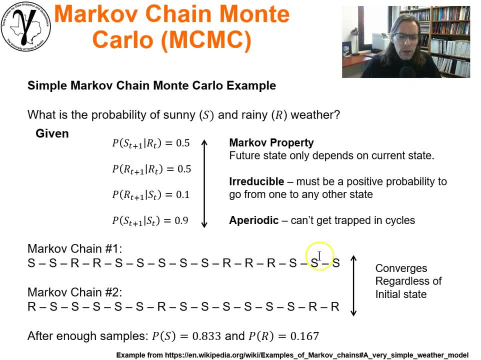 The probability of sunny or rainy. Now you could start another Markov chain, And often that's what people will do- is they'll have multiple Markov chains, So we'll start another one. It doesn't matter the state, We'll start it out as rainy and well. 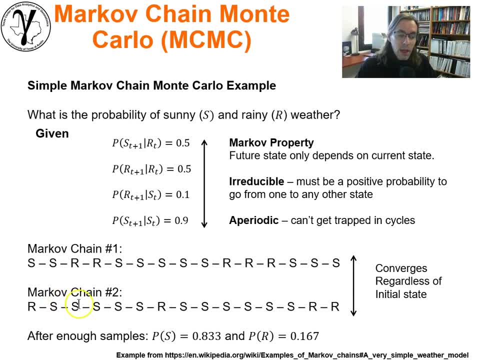 50% chance of sunny after rain. Okay, Sunny- 90% chance. sunny, sunny, sunny. lots of sunny, rainy- Oops, 10% chance of that happening. It happened Now. 50% chance to go back to sunny. 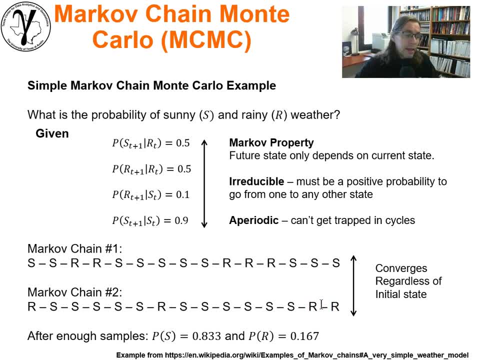 90% chance to be sunny, sunny and keep going. And so what we'll have is, after enough samples- we have enough samples of the of that global proportion of sunny and rainy- that we'll find out that it is about 0.833. 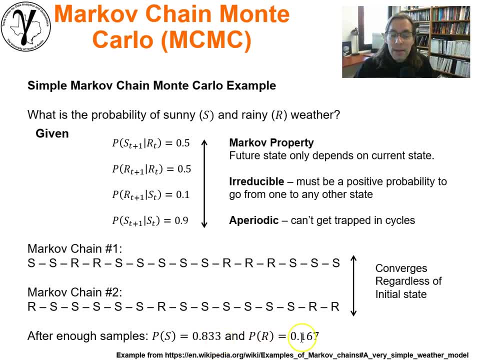 or 83.3% chance of sunny and 16.7% chance of being rainy. And we got to it by sampling that global proportion by simulating with Markov chains, Using Monte Carlo simulation Markov chains, because they're correlated. 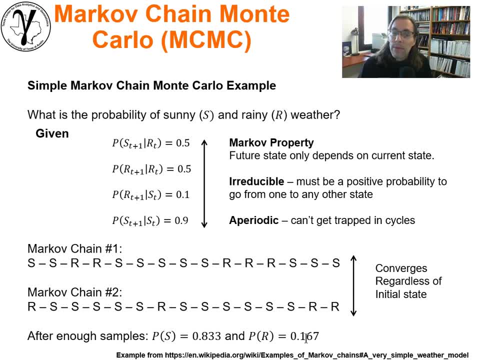 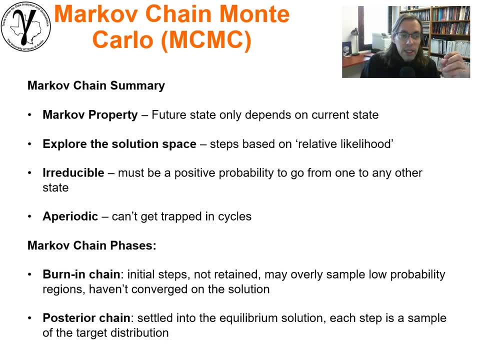 they're stepping through day to day. They have Markov property of only seeing the day before. They're really cool. Okay, So we got something really cool. Let's summarize what we've done. Markov chain summary um Markov property. future state only depends on the current state. 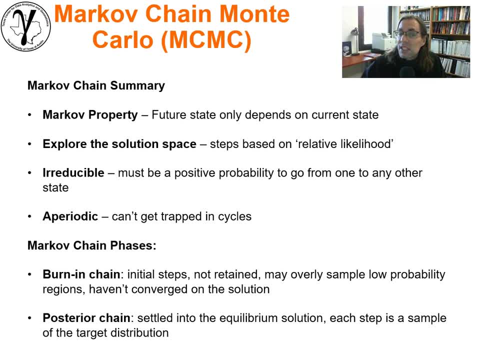 not the long history before we were able to step through and explore the solution space, knowing only the probability relative to the current state. Okay, Now if we were doing um, Metropolis, Hastings and other types of methodologies, we'd be working with relative likelihoods and so forth. 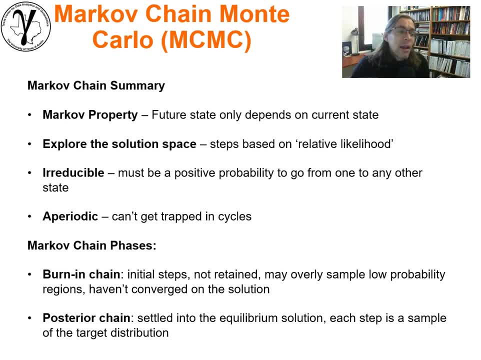 The main thing is that we step through in a way that is actually informed by the global proportion or the global distribution of the posture that we don't have. It knows it's proportional to its local density- Okay, It's a reducible in the 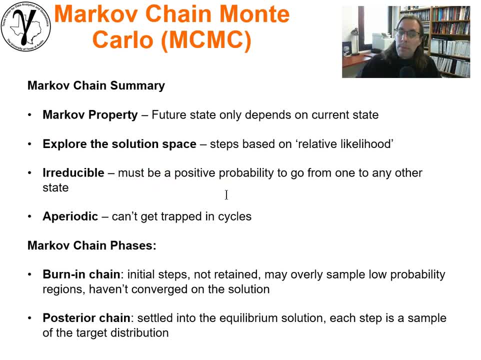 from the perspective that there is a probability of going everywhere, that we're able to explore the solution space. We don't get stuck. We don't get trapped in cycles either. Now you could note that if we had a much more complicated system, 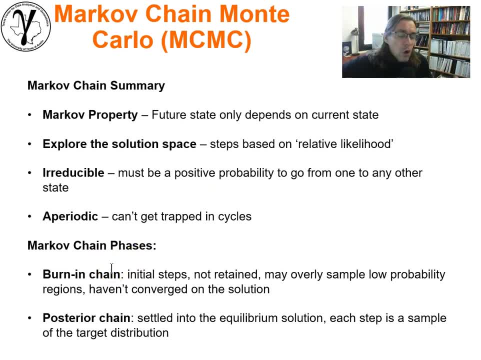 there's the chance that our first few steps aren't very good. That's what's known as the burn in chain, The initial steps. they're not retained. They may overly sample low probability regions. They haven't got to the really dense part of the probability distribution. 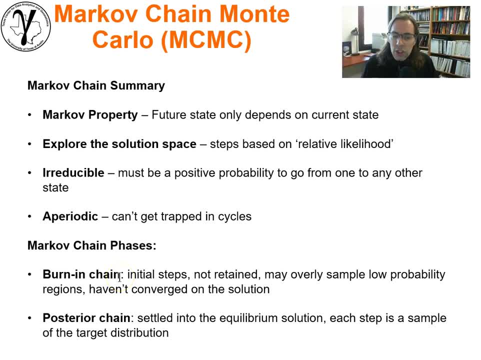 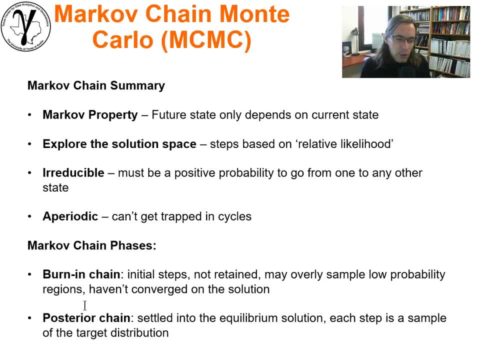 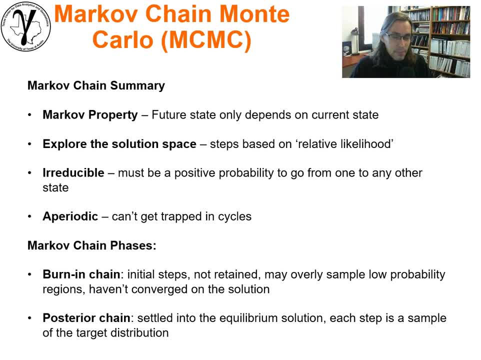 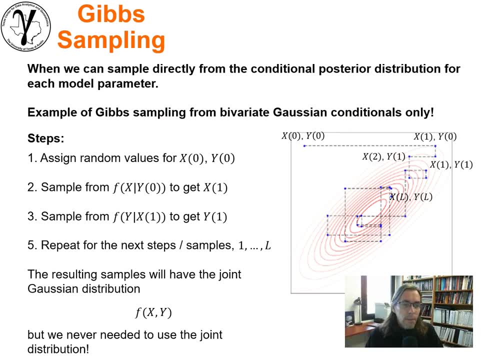 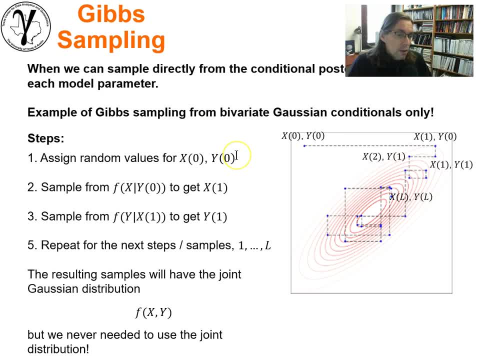 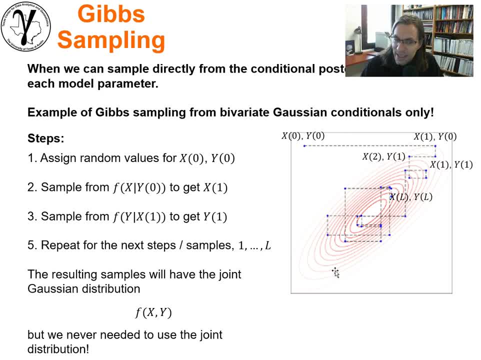 contours of what the bivariate Gaussian distribution density should look like. High density here, low density going out. We know the bivariate Gaussian, So assign a random value for x and y, So x, y and we got this value right here. That's not a very good value, It's not, It's outside. 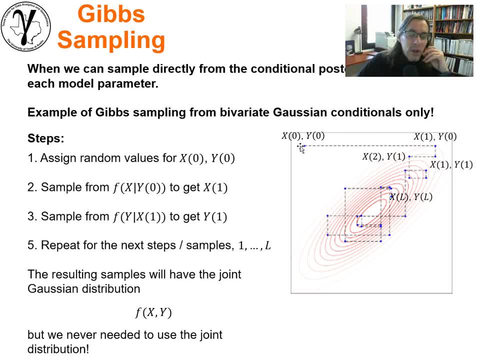 It's super low density. Probably shouldn't be there, right? What we do next is we sample from the conditional distribution of x given the y naught Okay. so if you calculate the conditional distribution of x given this y value, you'd find it's a distribution that goes like: 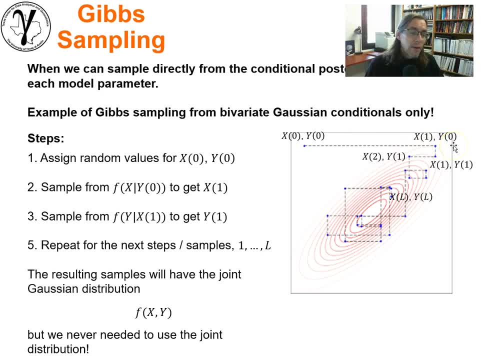 this Goes right there. So we draw a value from that conditional distribution for x. and now we have x1 comma y0 right here. So we've stepped all the way over here. Now we're going to sample from the conditional distribution of y given x1. So that conditional distribution drawn in this direction, would have: 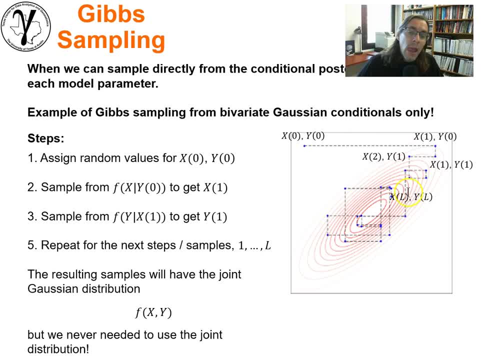 a bump like that, Its mode would be right around here. So we go ahead and we draw from it. We get this value right here, Repeat, repeat, repeat, repeat. You see what's happening here. And if we do this longer, we get this value right here. So we draw a value from that conditional distribution. 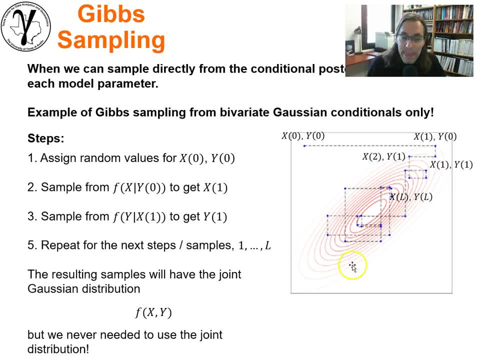 of y equal to x. Okay, this will have this value right here. So now we start to sample from the conditional distribution of x given x1.. Okay, So what we have to achieve is the Whilst: Oh, and this is how we go from the conditional distribution of x. Good enough. 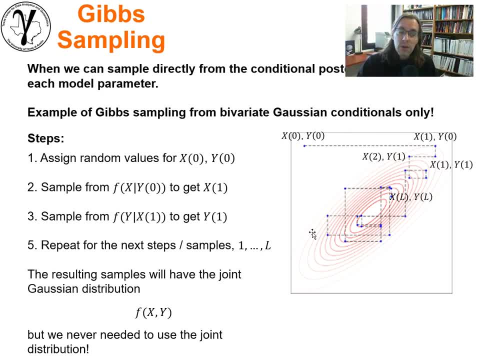 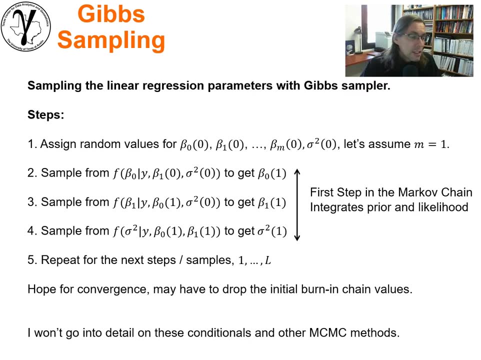 We will explore and sample the bivariate Gaussian distribution with densities of samples that are proportional to the actual densities of the target distribution. at no time that I even have to use the joint bivariate Gaussian distribution. I only need the conditionals. So how would we do Gibbs sampler for the purpose of the case of linear regression, the Bayesian linear regression? 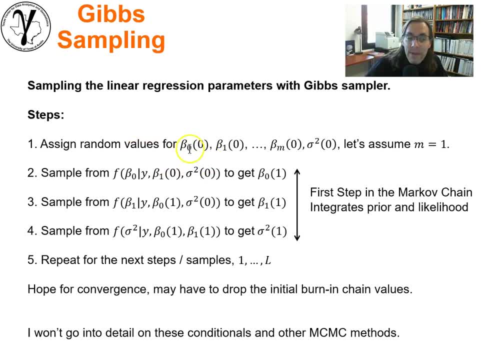 What we can do, then, is we can assign random values for the intercept, the slope, for each one of the 1 through m predictor features and also for the variance term right. Remember, we're modeling the entire distribution of uncertainty. We need to know the homoscedastic variance of the system. 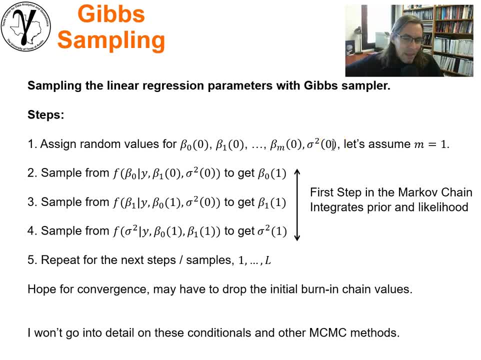 You remember we were applying it to the identity matrix before. Okay, so what we can do now is we go ahead and we'll, and as I step through here, I'm going to assume m is equal to 1.. I don't want to write out a bunch of stuff. 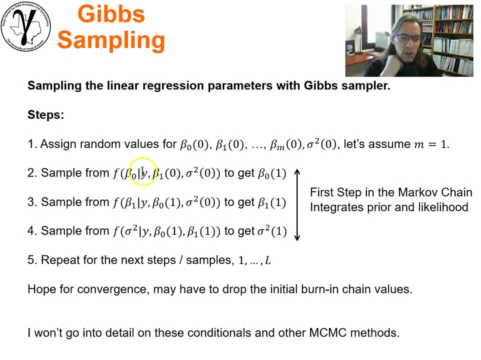 We can sample from the conditional distribution of the intercept term, given the y, x observations and all of the previous values of the previous. So that's the conditional we sample from. Now the good thing is for many distribution assumptions we know we can calculate these conditionals. for some problems. 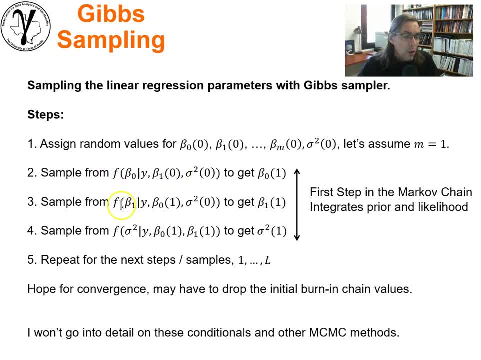 And so we just have the conditionals available to us, We can go ahead. and then we sample for the slope term, given that intercept term we just got, Then we sample for the variance term, given that, and then repeat, repeat, repeat, repeat. 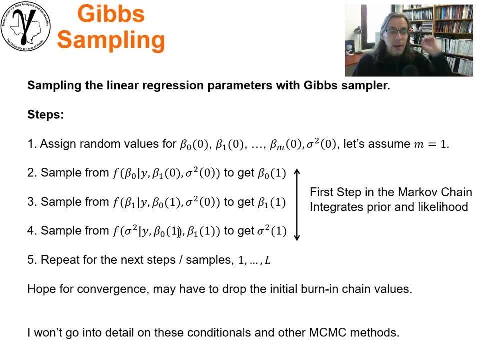 And so what's happening here Is, by the time we've got here, we've actually got one sample for every one of the parameters, And so this is really powerful. We're counting for their correlation structures with regard to each other. We're sampling from this very difficult posture. 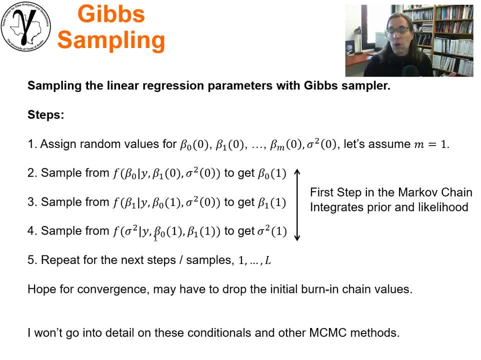 And we just repeat that one time, two times, three times, all the way up to L, and we'll get L samples. Now we could check the trace plot, as I'll show you, and we could check to make sure that we don't have burn in chain. 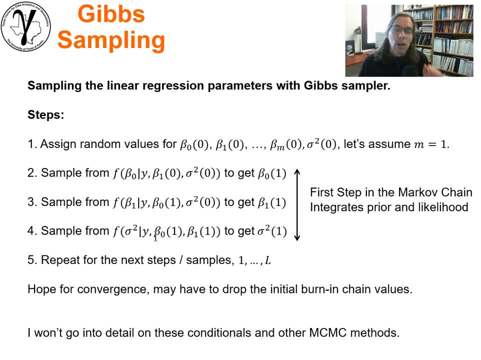 If we do, we have a different behavior in the parameter. So up front we chop that off and we start working with the posture chain where things have started to stabilize again into that equilibrium that's matching the target. Now I'm not going to go into any details about these conditionals for the purpose of Bayesian linear regression. 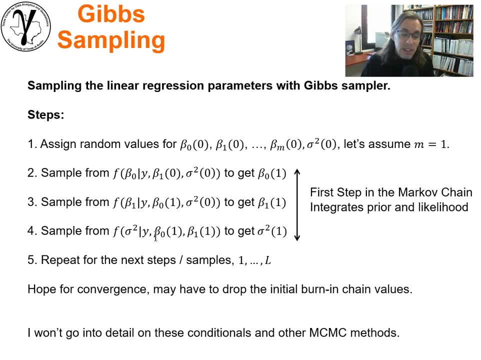 We could teach an entire course on Bayesian methods specifically around this. There's a lot of theory we could get into, I think, for the purpose of this class. this was enough to talk about as far as Markov chain, Monte Carlo Simulation as a methodology to solve Bayesian types of machines and sample from the postures, 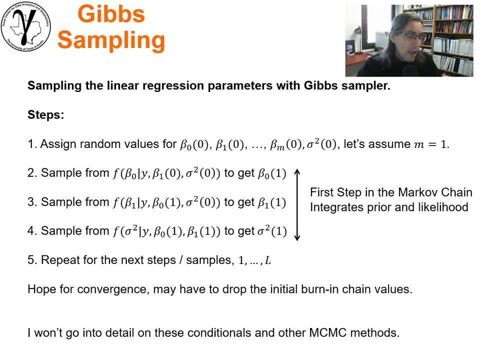 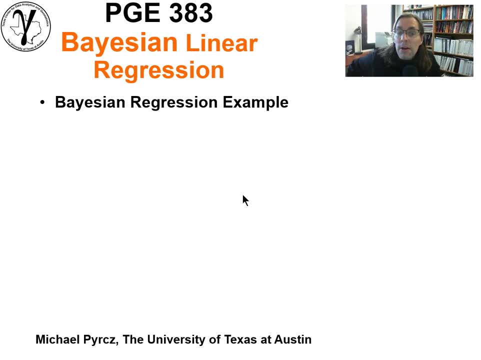 I think that was sufficient for now, and I hope that you found it helpful Now. next, what I'll do is I'll provide a Bayesian linear regression example and that'll be in the next lecture. All right for now. thank you very much for listening. 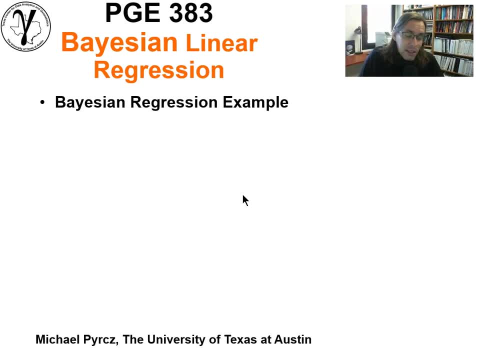 I'm Michael Perch. I'm an associate professor at the University of Texas at Austin. It is my joy and pleasure to share data analytics and geostatistics machine learning with anyone who wants to learn about it. In fact, to the point that I spend time recording every single one of my lectures that I teach in the university here. 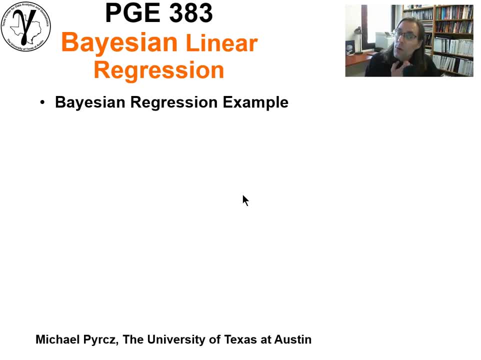 and I provide them to anyone in the public. I'm so excited I get great feedback from professionals working in my industry in the subsurface and development- and keep sending me happy messages and letting me know if this is helping you. I am like a DJ here. 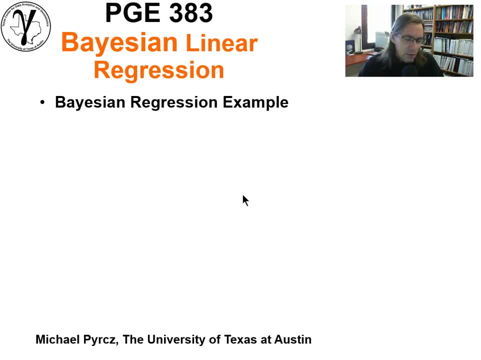 If you send me a request, I may actually play your song, So let me know if there's something else you want to hear about, If you have feedback. it's all about sharing knowledge, All right, thank you very much for attending. Okay, bye. 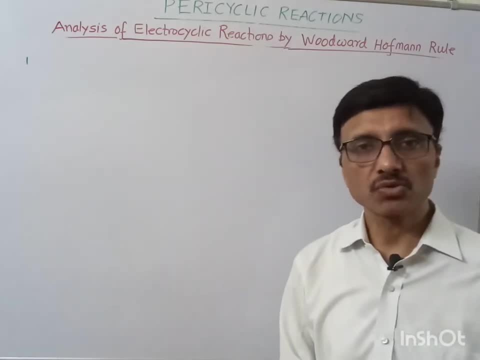 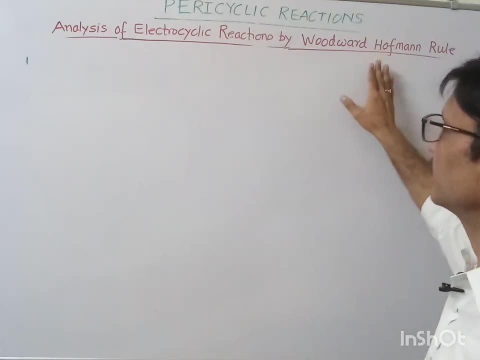 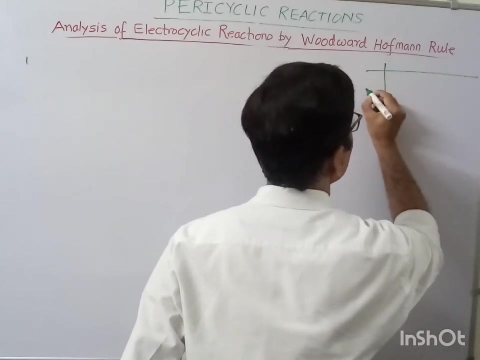 method and Huckel-Mobius method, or also called as the PMO method. So let us see its analysis. analysis of electrocyclic reactions by Woodward Hoffman tool. So already I have told you the rule, selection rule for this electrocyclic reaction, that is, for two type of electrocyclic reactions.